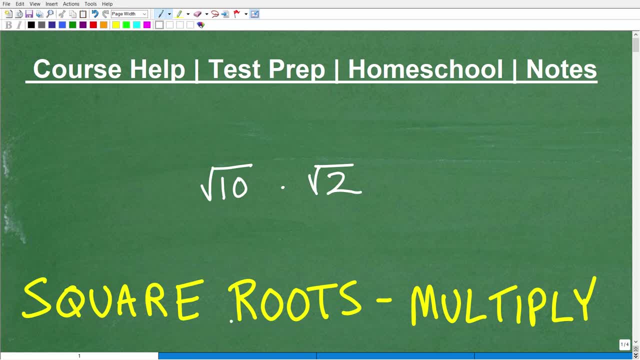 Okay, let's talk about how to multiply square roots. That is the topic of this video. This is going to be just a quick power lesson on square roots and how to multiply. So I got a couple examples, but you just don't want to. you know, see my examples here and be like: okay, I understand, this is all I need to know. You want to practice this stuff. So, when it comes to square roots and algebra- and this is kind of the stuff you learn in algebra- it's very, very important that you get really comfortable with this Now when you're. 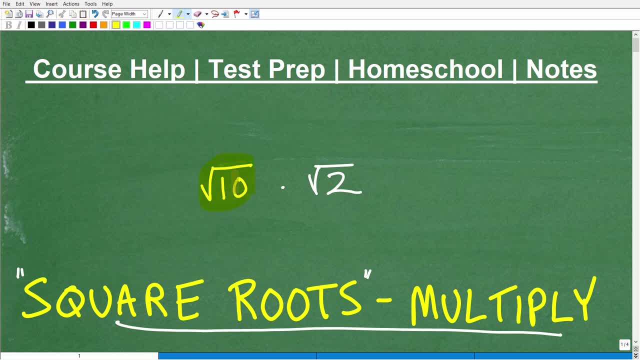 what we're definitely not talking about is: oh okay, I can go into my calculator and take the square root of 10, I get some sort of decimal that I multiply by the square root of two by going into my calculator and taking the square root of two. that's not what we're talking about here. So we want to put our calculators away And you'll see exactly what I'm talking about, But this is absolutely essential in terms of algebra and working with square roots, etc. So we're going to talk about some of the main principles here. 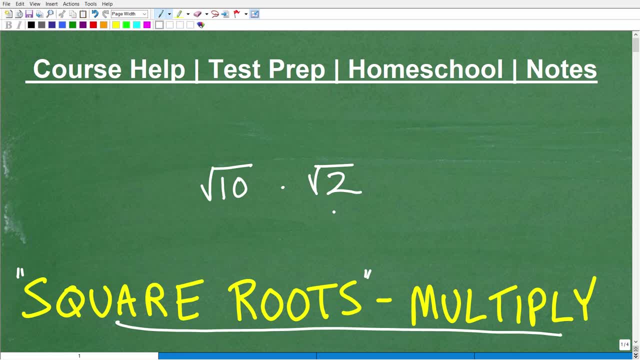 Multiplying square roots is not that difficult. But you know there's some follow on steps that if you don't do you will not get the problem correct. But if you think you could do this problem, go and pause the video and put your answer in the comment section. I know you can't make a square root symbol, but maybe you could just put in square root. you know something like that. You know use that as a little abbreviation for square root. but you can definitely express your answer. if you think you can get it right, Put that into the comment section and we'll get to that. 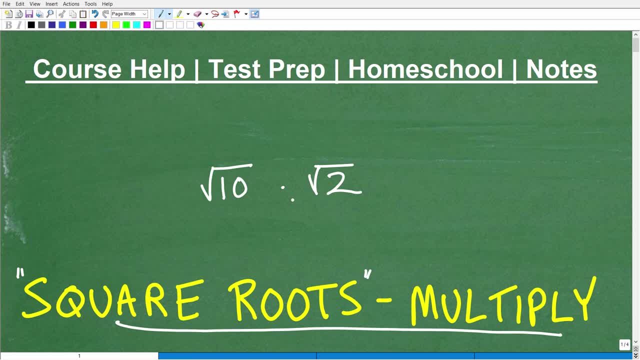 So I'm going to put a little pair of notes here in just one second. But first let me quickly introduce myself. My name is John. I'm the founder of Tablet Class Math. I'm also a middle and high school math teacher. I'm going to leave a link to my math help program in the description of this video. But if you are having a tough time in math, or maybe you really want to get ahead in math- whatever the case might be- maybe you don't feel like you're getting the right instruction or you don't connect with your teacher's teaching style. whatever the case might be, I've been teaching math for decades And my style of teaching is: I like to break. 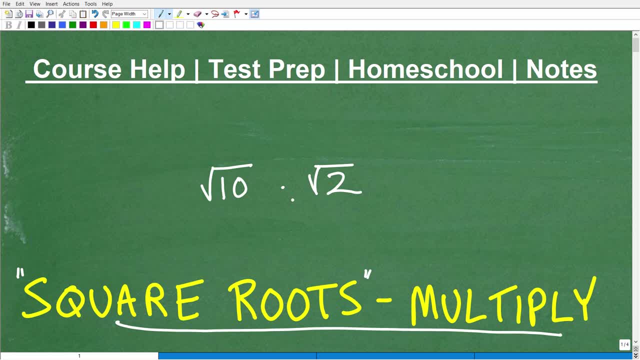 concepts down into very bite-sized, clear and understandable components so everyone can learn this stuff. So if you really feel like you, you know, are not capable of learning math or you just naturally have a tough time learning, that doesn't have to be the case. What you need is a. you need clear and understandable instruction and you need a lot of it and a lot of practice. So if you're willing to work hard at it, you know, coupled with good instruction, you can be successful in math. So if you're at the middle school, high school or even college, 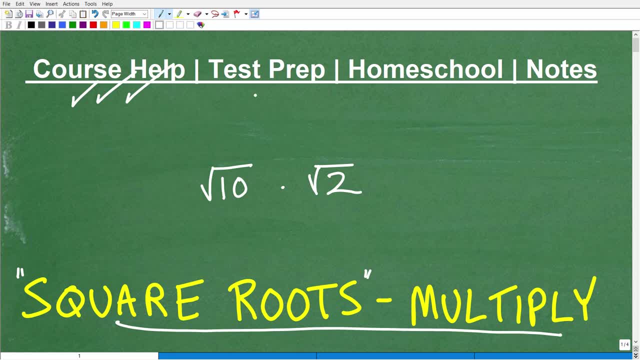 in terms of mathematics. I can definitely help you out Now if you're preparing for some sort of test that has a math section on it. so I'm talking about things like the GED, SAT, ACT, GRE, GMAT, ASVAB, ACCUPLACER, CLEP exam, teacher certification exam, nursing school entrance exam. There are so many exams out there that people have to take for all sorts of reasons that have a math section on them. I can help you prepare and pass those exams. If you homeschool, you absolutely must check out my homeschool math. 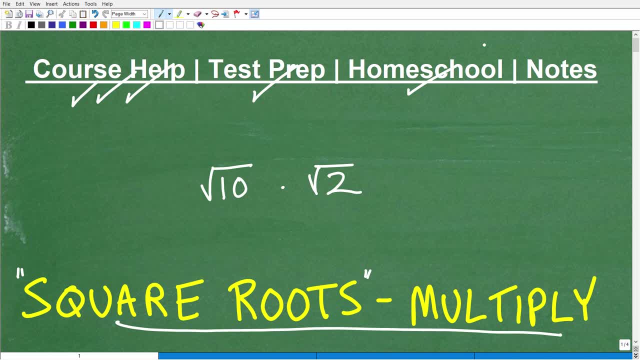 program and courses, full curriculum, everything you need to be successful in homeschooling. And if you don't have any math notes to study from, you can use mine. I'm going to leave links to my math notes in the description of this video. But if you want great grades in math, you must take excellent math notes. So start improving your notes and you'll see your grades start improving right along with them. So let's talk about square roots. So how do we do the square root of 10 times the square root of two? Well, I'm going to show you this in just one second, But first let's 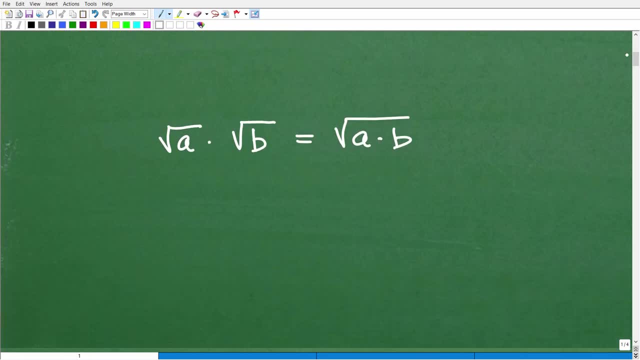 quickly talk about the whole property here. Okay, so this is the property you need to know. in algebra, the square root of A times the square root of B is equal to the square root of A times B. Okay, so this is what we want to understand. So when we have two individual square roots, okay, we can. these are the numbers, by the way: A and B. So the square root of A times the square root of B is equal to this one big square root of A times B. So we want to interpret. 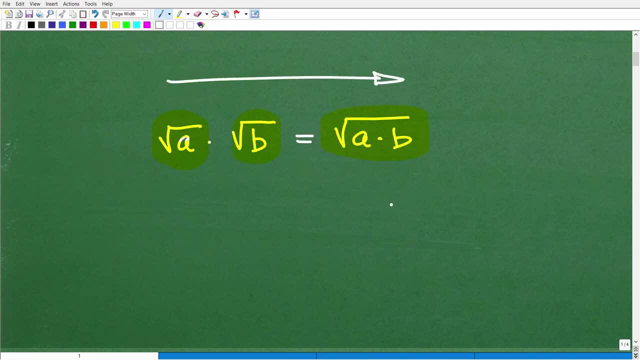 this property going this way And we also want to interpret the property going this way as well. Okay, so, in other words, if we look at this square root of A times B- in other words, I can write it this way- the square root of A times B is equal to the square root of A times the square root of B. Okay, so what is A times B in this case? Well, this would be factors of a number. Okay, I'm going to show you why this is really, really important here in a second. But this is the property that you 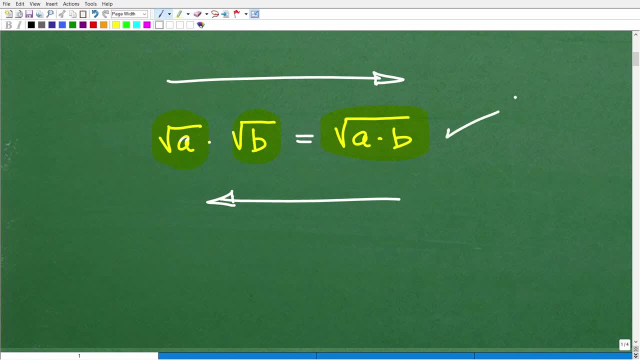 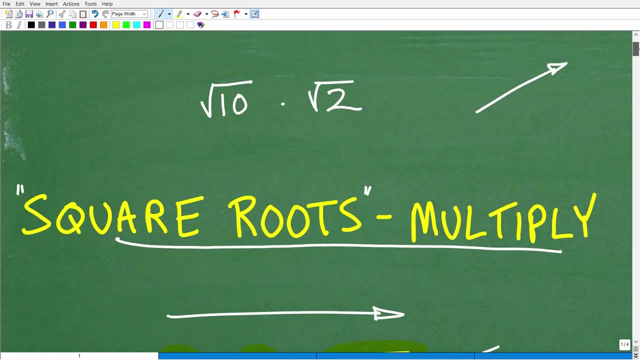 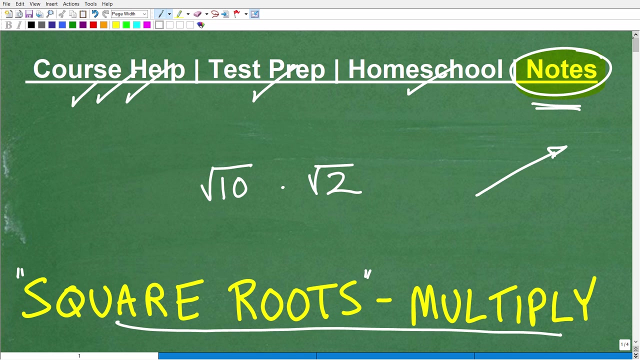 need to understand. Okay, and hopefully you do understand that. Now let's go back to our problem. the square root of A times the square root of B is equal to the square root of A times B. So here is the problem again. Now you know, I've kind of given you the path forward to how to get. 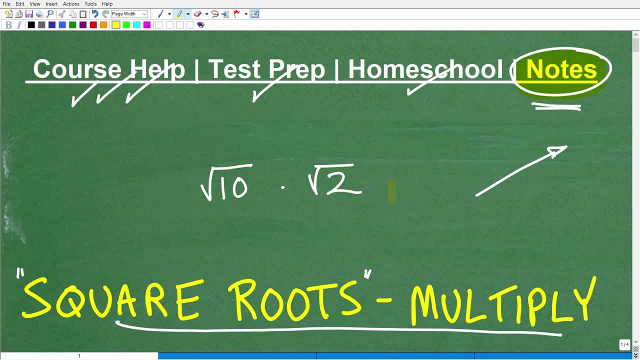 this right. So what is the answer? Okay, what is the correct answer now? So, how many of you think the correct answer is the square root of 20? Okay, well, if you said the square root of 20, oh, it's a square root of 20.. That's the- you know an application of that property. Well, 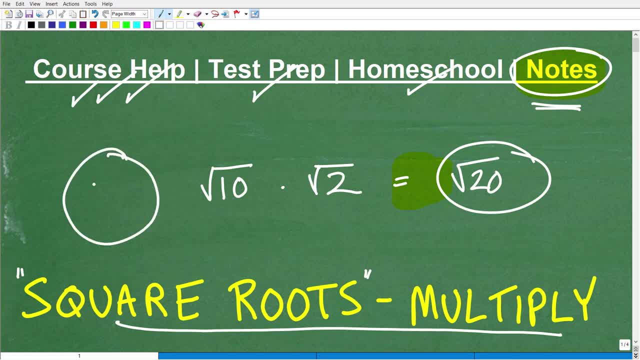 I would say: are you finished? Okay, because if you are done, I'm kind of have to give you a little bit of a sad face. Okay, you're like, what are you talking about? Maybe your hair is like this. 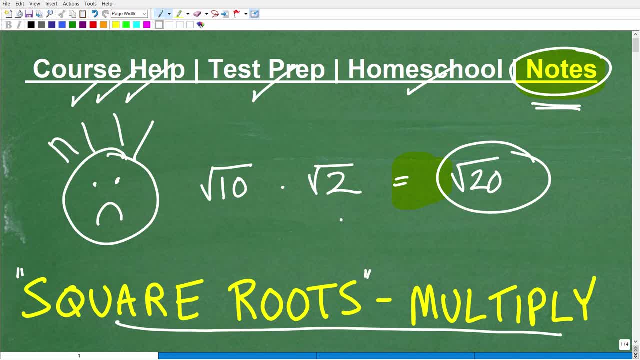 you just told me what to do, Why you're saying the square root of 20 is wrong. Well, this is not fully simplified. Okay, so you want to finish this problem? I said: are you finished? Okay, so finish this up if you know how to finish this up, So we can get you a nice little happy face. 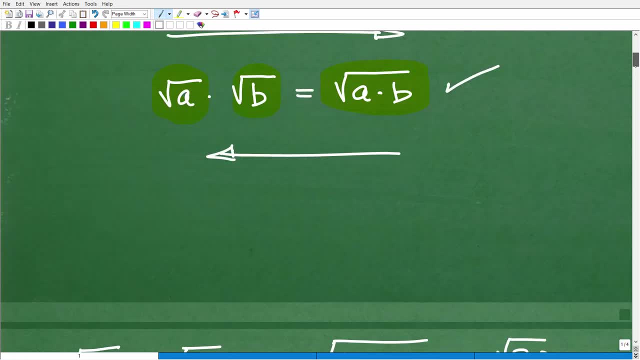 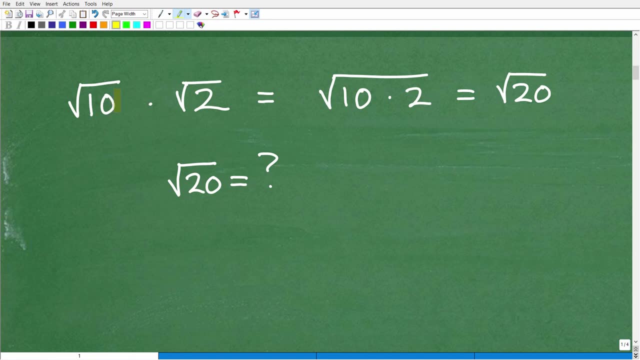 here, But let's talk about this specific problem And we'll do another example Again. you're going to want to practice this stuff beyond these quick examples, Okay. so here we got the square root of 10 times the square root of 2.. We're following this property. okay, the square root of A times. 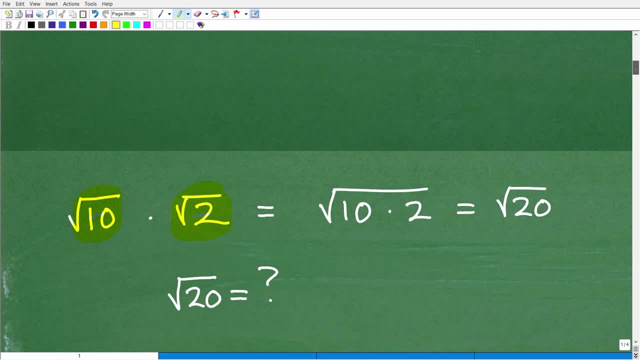 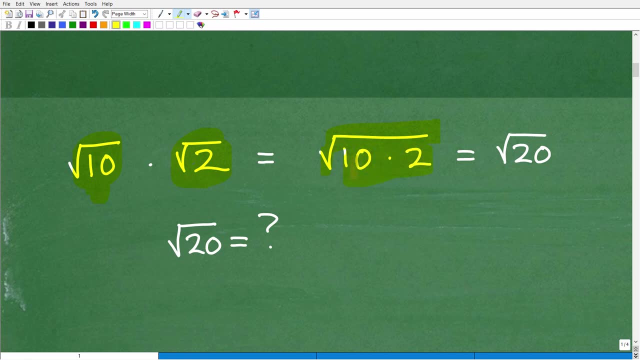 the square root of B. We just write one big square root of A times B. So when we follow that, this is one big square root. Here's our A, here's our B: 10 to 2.. So we're talking about the square root of 10 times 2,. 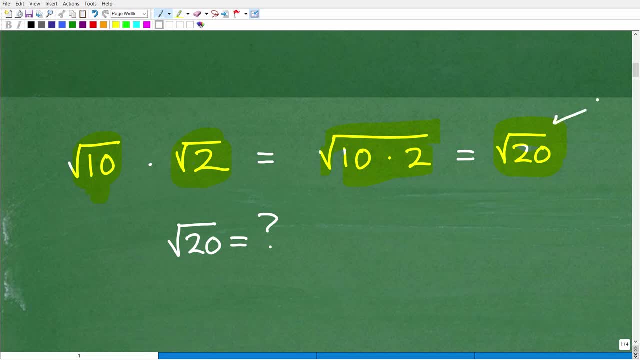 which is the square root of 20.. So this is good. Okay, but we're not done yet, All right. So in algebra, when we're dealing with square roots, you want to simplify. Okay, and your teacher's not going to be happy if you give them this answer: the square root of 20.. They expect you. 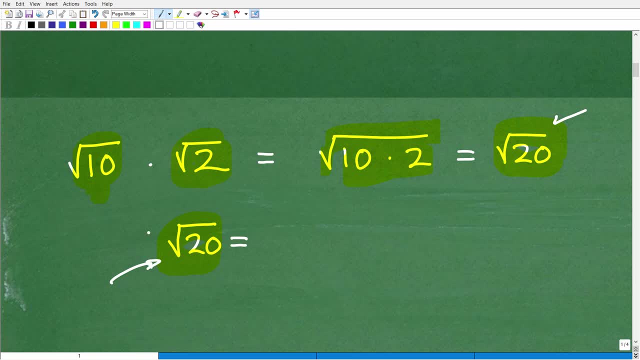 to fully simplify these square roots and radicals. Okay, so how do you do this? Well, I'm going to give you a couple of suggestions. If you don't understand how to simplify square roots, I have tons of videos on my YouTube channel: my pre-algebra and algebra playlist. Of course, I teach this. 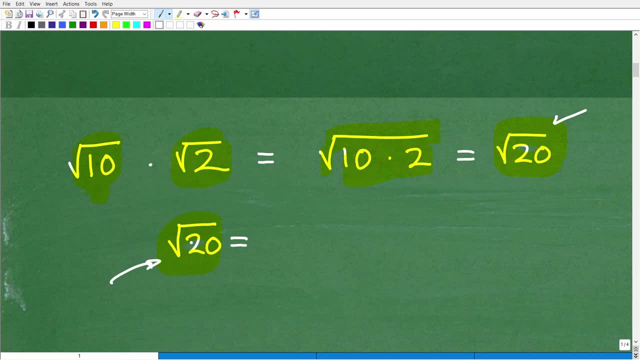 extremely thoroughly in all of my algebra courses. but let's talk about how we can simplify All right. so real quick. what you want to do is look at 20 and try to think of two numbers that factors of 20, and you want to be looking for factors, what we call perfect squares. So 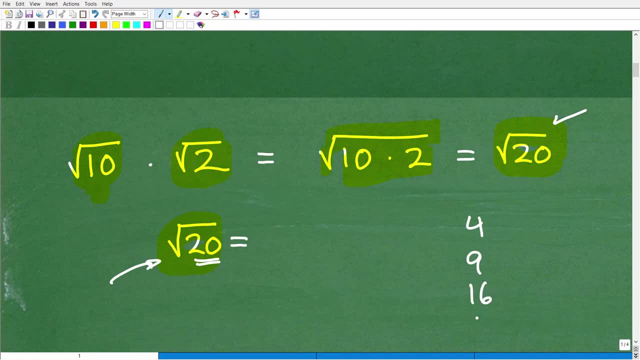 things like 4, 9,, 16,, 25, there's a ton of these type of numbers, an infinite amount of numbers that are perfect squares. Now, why are these called perfect squares? Well, because when I take the square root of these, and we're talking about the principal square root, we don't have to worry. 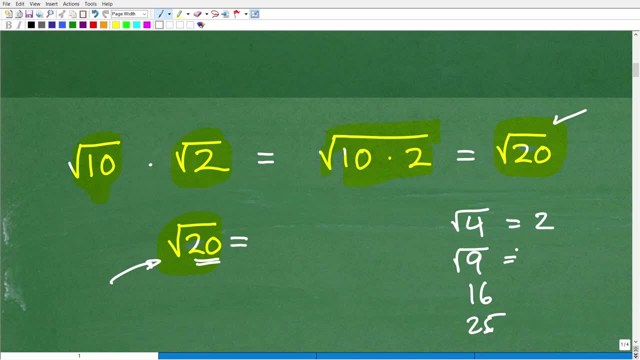 about the positive, negative part, although you need to understand that as well. We get these nice lovely numbers like so, Okay. so these numbers 4, 9,, 16,, 25, etc. These are what we call perfect squares, Okay. so when I look at 20, I'm like, hmm, oh yeah. 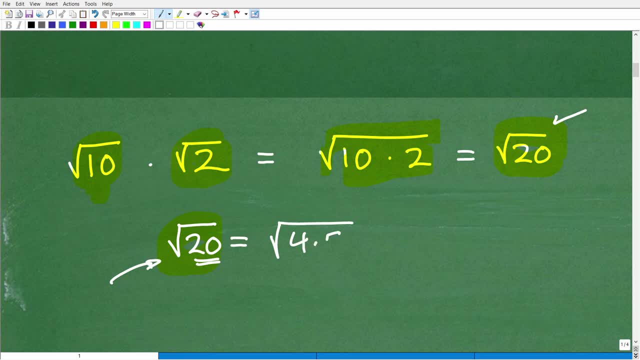 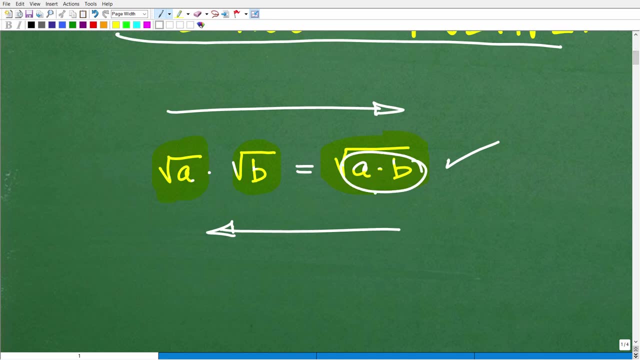 there's a perfect square in there, it's 4.. So I could write 20 as the same thing as 4 times 5.. So remember I was talking about. you can go this way. I can write these fact. I can write a number. 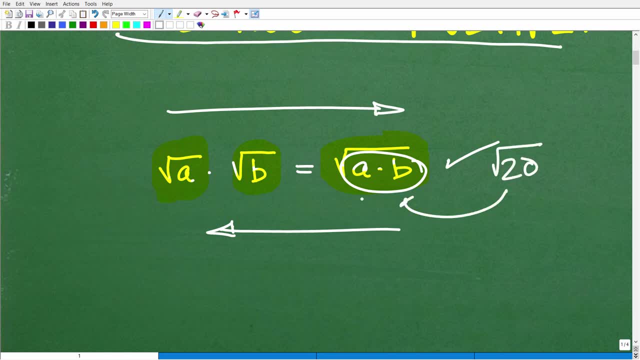 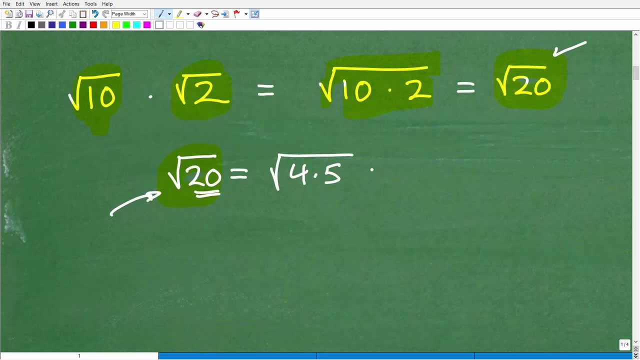 like 20 in terms of its factors, which would be 4 times 5, and now I could split this up in its component parts. Okay, this is kind of like doing the exact reverse. Instead of going this way, now we're going this way. So the square root of 4 times the square root of 5, I can break up. 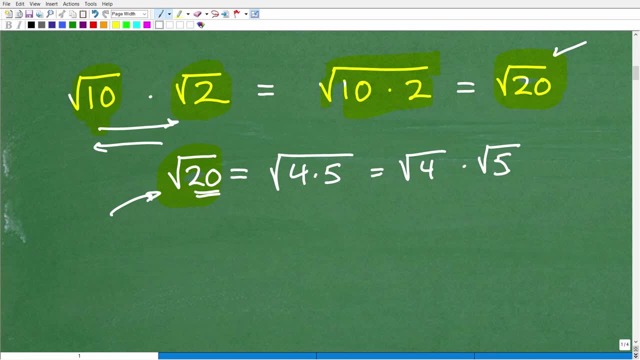 like this: square root of 4 times the square root of 5.. And of course, I just you know, if I gave you this as a problem, you'd be: oh, that's the square root of 4 times 5, or square root of 20.. 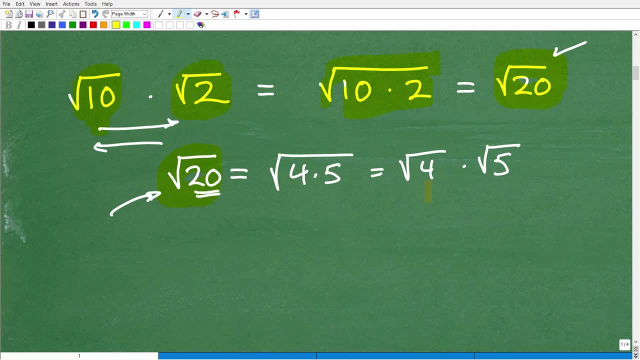 But what's the advantage here of writing it this way? Well, I have the square root of 4, and now I know the square root of 4 is 2.. So this is 2 times the square root of 5.. So just a quick. 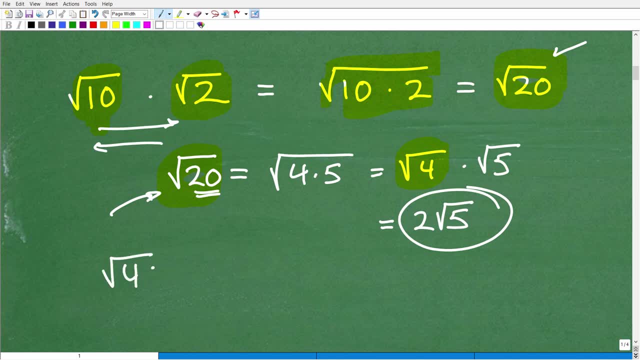 review here. The square root of 4 is 2, but it's also- you can think of it as negative- 2.. But anytime you're working with square roots and whatnot, it all depends on the situation. If you're working with equations, you're going to need to know that the square root of 4 is both. 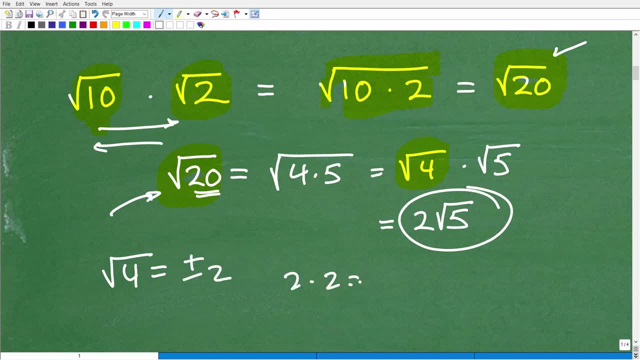 positive and negative 2,, because 2 times 2 is 4, and negative 2 times negative 2 is also positive 4.. So these are both correct. However, when we're working with problems and it's not really explicit in terms of an equation, 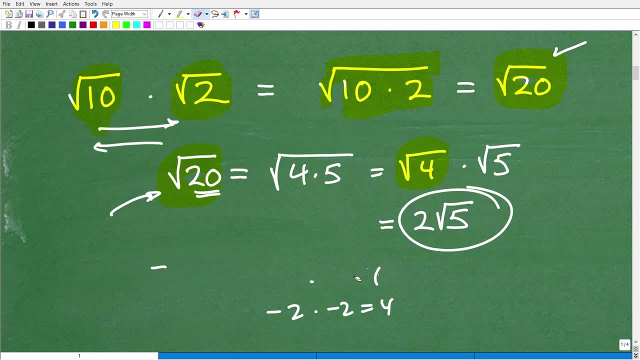 or something like that. it's okay if you just write what we call the principal square root, It's just the positive part of that square root. So the square root of 4, we can just write as 2, positive 2 times the square root of 5.. And this is the final answer. So if you got that right, 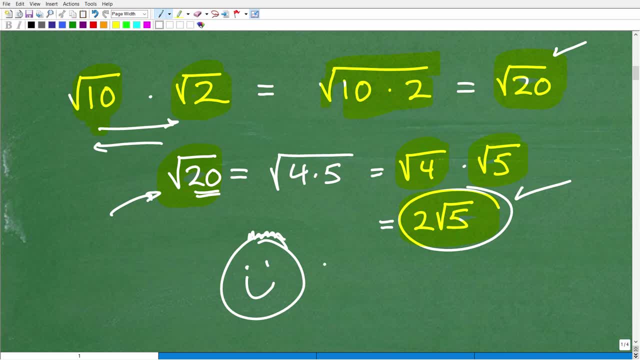 then I must go ahead and give you a nice little happy face with a good old 1985 laptop haircut. Nice job, Okay, All right. So let's go on and take a look at another problem, and then we'll wrap this up. 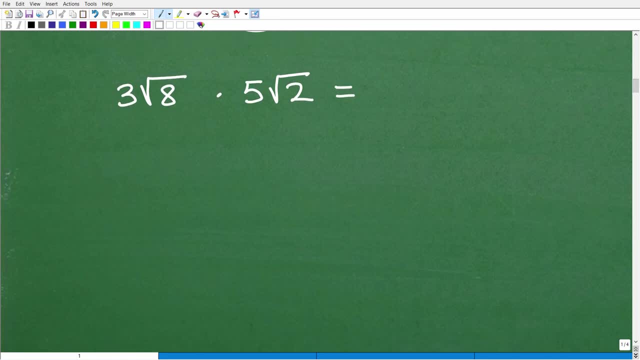 again, This is not enough practice to say, oh okay, I'm an expert in square roots and everything else and radicals. That's one of the worst things that math students do Here. let me just show you real quick. So let's say, this is your homework and you have, let's say, 20 problems assigned. 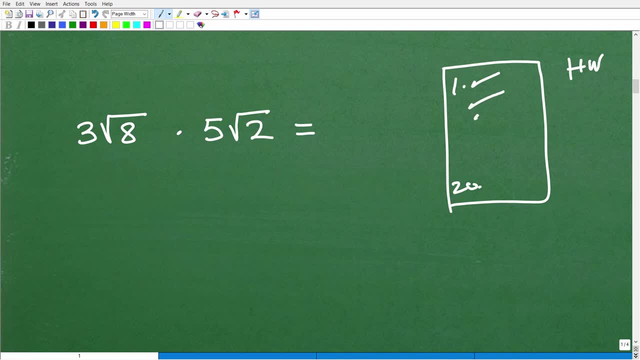 And you're like: oh, I got number 1 right, number 2 right, number 3 right, number 4.. I'm like, oh man, I'm getting all these right. I must be an expert. So guess what, I don't have to do the rest of this stuff. It's a waste of my. 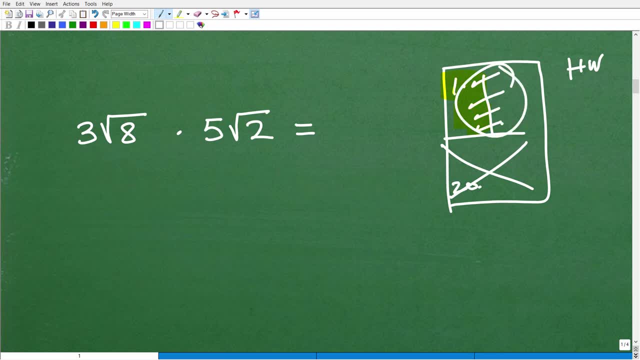 time, because I've already proven to myself that I know what I'm doing. That's wrong, wrong, wrong, wrong, wrong, Okay. Typically, this is like the easy and more basic problems. You need all these problems. You're trying to, you know, establish a math skill- Okay, Mathematics in all its little. 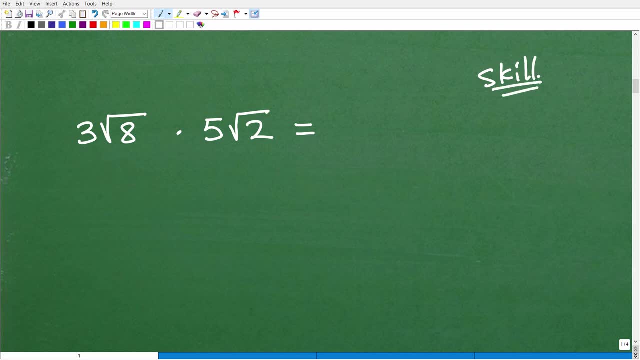 parts is a skill Like what would be an example of a skill like in sports. Well, shooting a basketball is a skill, or throwing a baseball or hitting the baseball or any type of thing. That requires a lot of practice And the more you practice, the better you're going to be. 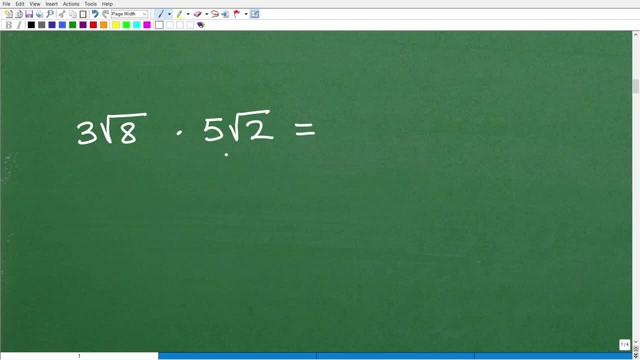 at it. So math is no different. Okay, So let's take a look at this last problem here. So we're talking about multiplying square roots, So how do we do this one? Well, we have 3 times the square root of 8, times 5 times the square root of 2.. Go ahead and see if you can figure this out. Put your 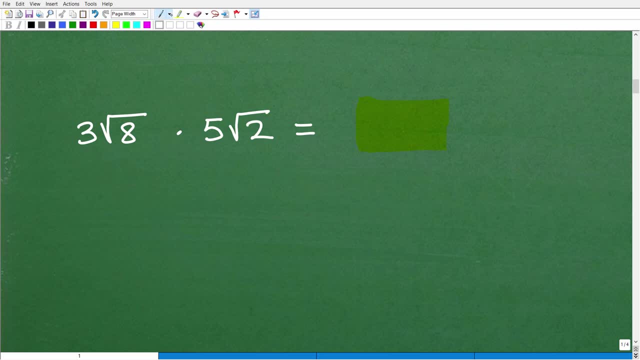 answer right in that comment section. But if you don't want to see the answer, go ahead and pause the video and work on this for a quick second. But let's go ahead and talk about how we're going to do this, All right, So here this. 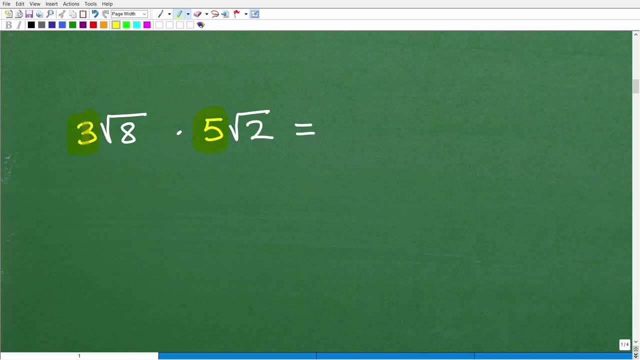 is a number and we're going to multiply it by this number. Okay, This is. this number is being multiplied by this And this is all being multiplied together. In other words, we have 4 things being multiplied: 3, 3 square root of 8 means 3 times the square root of 8 times 5 times. 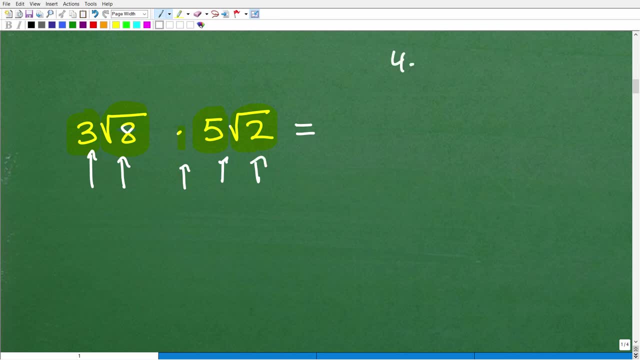 the square root of 2.. So I can rewrite: if I said 4 times the square root of 2, I can multiply it by this number. So uz times square root, 2 is 6 times the square root of 8 is 6 times the square root. 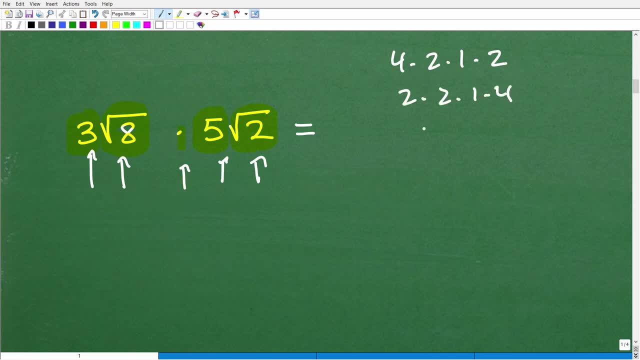 of 8.VE. All right, So how the number does it work? If I said 2 times the square root of 18, times the square root of 20,, if I had just put my umbilical number, you could. 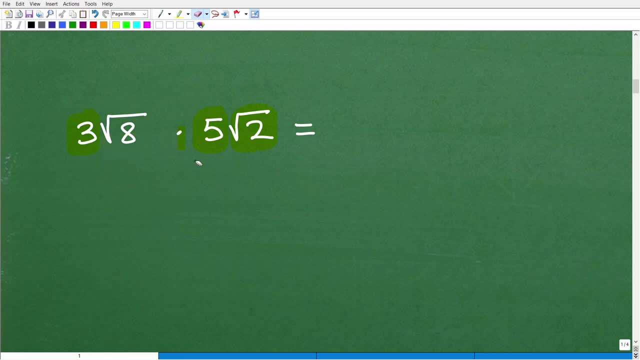 know. Okay, so how do we got the close number? What happens when we multiply? What happens when two you add? now you know, Do you notice that you? let's write it? just write it out here. so this could be three times five. you're going to do the. 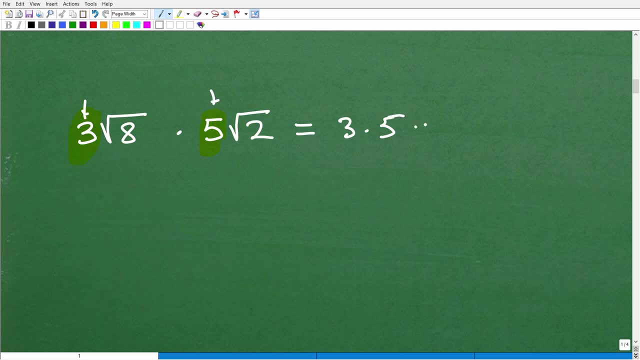 number parts right here, and then we could have square root of eight times the square root of two. okay, so this is a equivalent. this right here is equivalent to this. i just kind of put things in different order, so i can multiply the three and a five. of course that's going to be 15.